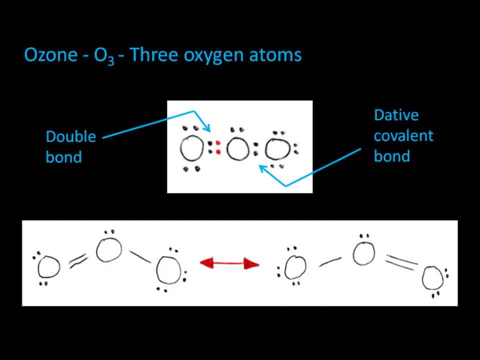 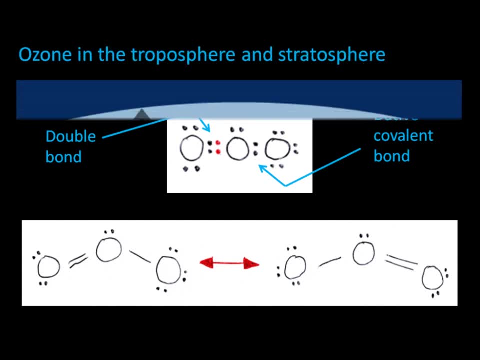 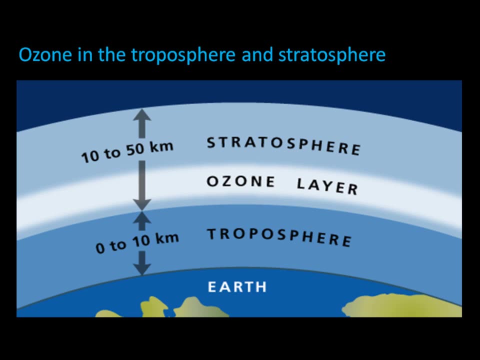 see there is one double bond and one coordinate or dative covalent bond. Let's look at where the ozone is based within our atmosphere. Ozone is in the troposphere, based seven kilometers above the poles and around 20 kilometers above the tropics. Here it is an air pollutant and poses a threat to animals. 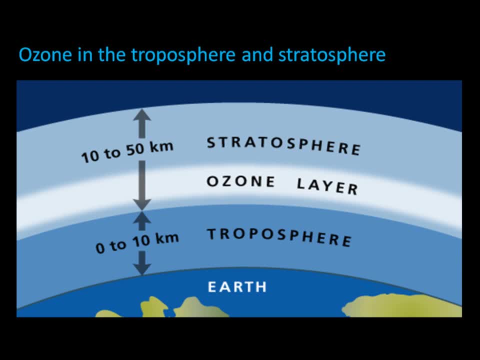 and plants. Ozone is mainly seen in the stratosphere, based 10 to 50 kilometers above Earth's surface. This layer of ozone protects living organisms by preventing harmful UV light from reaching the Earth's surface. The ozone layer found in the stratosphere. 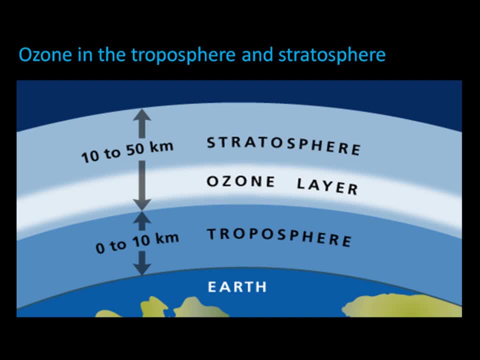 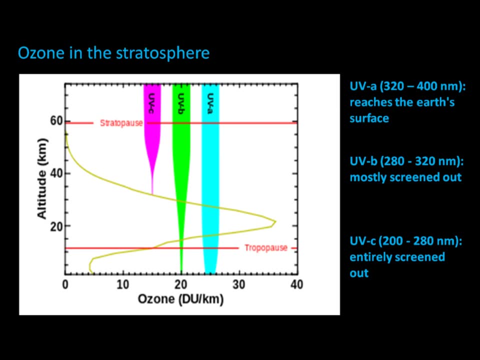 filters out the shorter or high energy wavelengths of UV light emitted by the Sun. This is shown here. UVA with a wavelength of between 320 and 400 nanometers. This reaches the Earth's surface. The UV radiation is relatively low in energy and does not cause much concern. UVB with a wavelength of between: 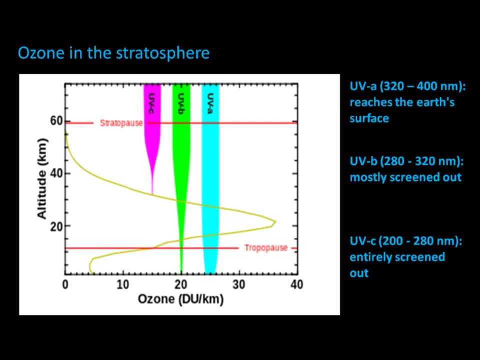 280 and 320 nanometers. This causes sunburn and genetic damage if exposed to, for a prolonged period of time, UVC with a wavelength of between 200 and 280 nanometers. This is entirely screened out by the ozone layer. Although ozone screens out most of UVB, some 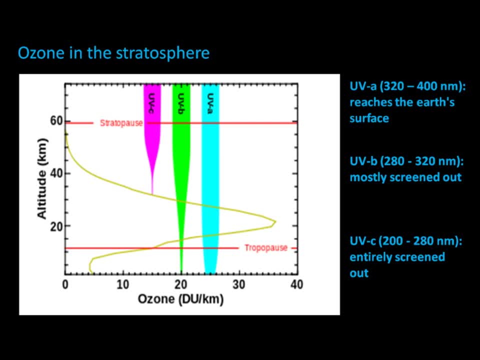 does reach Earth's surface. Any decrease in the ozone layer would allow more UVB radiation, which would cause more UVB radiation to reach the Earth's surface. Any decrease in the ozone layer would allow more UVB radiation to reach the Earth's surface. Any decrease. 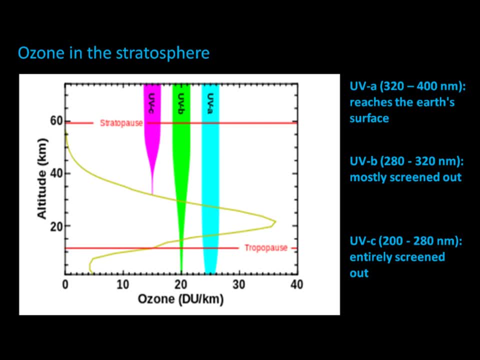 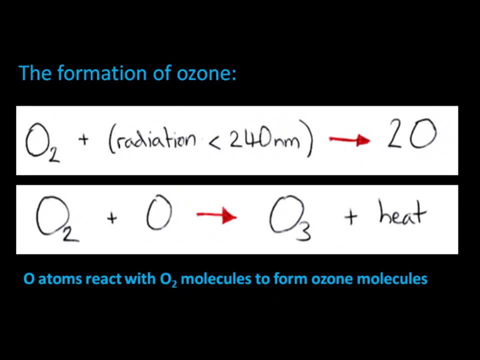 in the ozone layer would allow more UVB radiation to reach the Earth's surface. This is highly problematic. Firstly, let's see how ozone is continuously being formed and broken down in the stratosphere. through a natural equilibrium, The formation Oxygen molecules absorb high energy UV radiation less than 240. 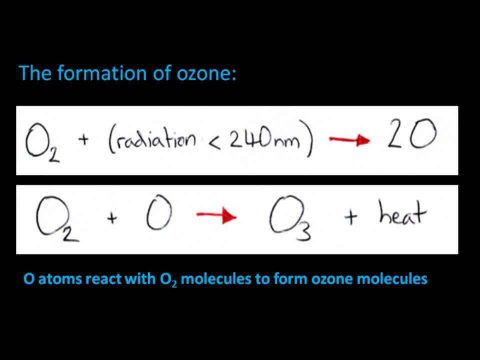 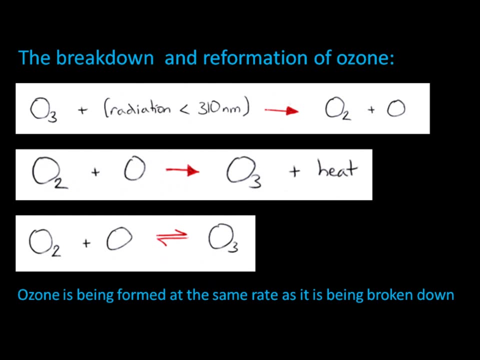 nanometers. This is capable of breaking the oxygen molecule into two oxygen atoms. This atoms, The oxygen atoms, then react with oxygen molecules to form ozone molecules, and heat is given off The breakdown. The ozone molecules formed in the reaction on the previous slide then absorb UV radiation with a wavelength between 240. 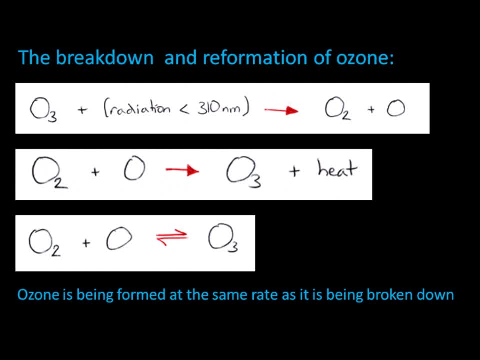 and 310 nanometers. Ozone is broken down. The oxygen atom produced immediately reacts with another oxygen molecule to reform ozone. This cycle keeps the ozone layer in a stable balance. A state is reached where ozone is being formed at the same rate as it is being broken down. There is an equilibrium Removal of ozone. 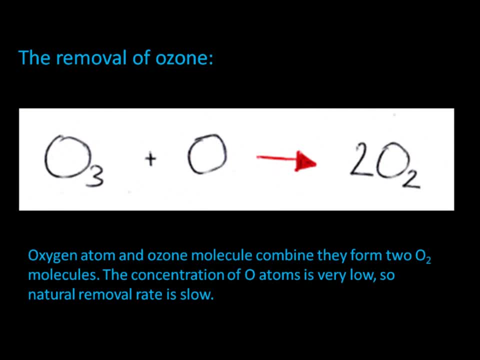 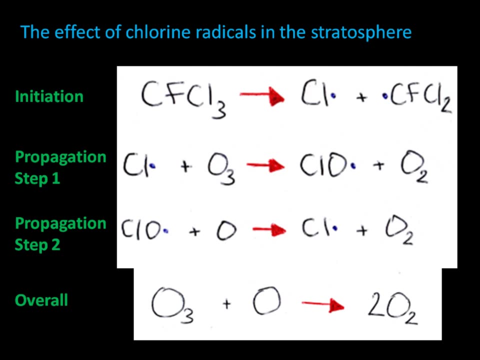 When an oxygen atom and ozone molecule combine, they form two oxygen molecules. The concentration of oxygen atoms is very low, so the natural removal rate is slow. It is our contribution to the ozone that poses a threat in terms of ozone depletion. Chlorine radicals in the 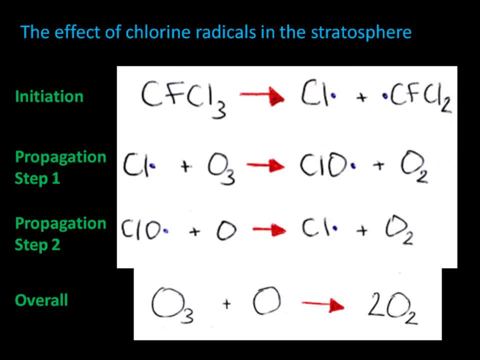 stratosphere disrupt the natural equilibrium of ozone formation and breakdown and are generally generated through human activity. They originate from the presence of chlorofluorocarbons, or CFCs, that have reached the stratosphere. CFCs are highly stable. Chlorofluorocarbons are highly stable. Chlorofluorocarbons are highly stable. CFCs are highly stable. 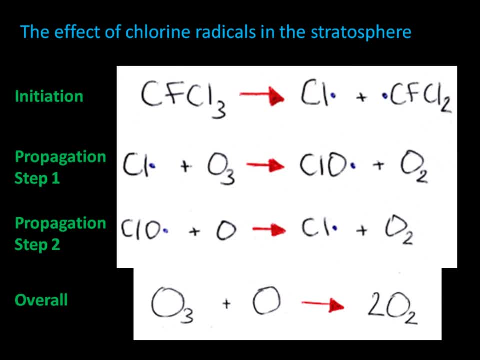 Chlorofluorocarbons are totally stable and can only be broken down by the extremely energetic UV radiation found above most of the ozone layer. It can take up to 30 years for a CFC to reach the stratosphere. When UV strikes a CFC molecule in the stratosphere. 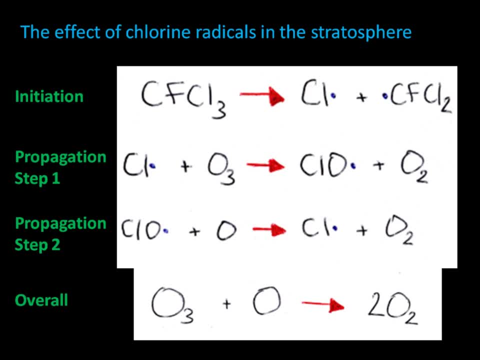 a carbon to chlorine bond breaks, producing a chlorine radical. The reactivity of this radical is high and is responsible for propagating the breakdown of ozone. As you can see here, in the second propagation step the chlorine radical is formed and will go on to attack another ozone molecule. 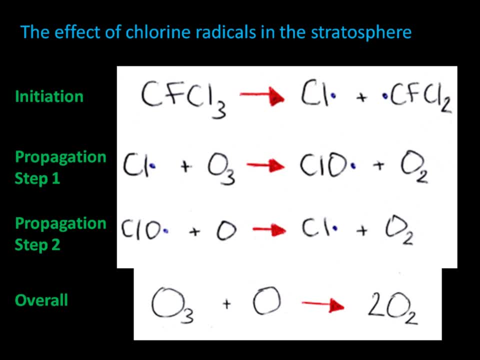 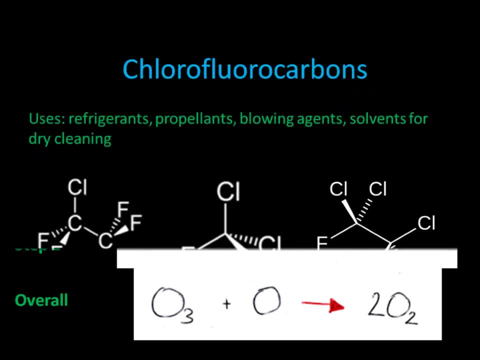 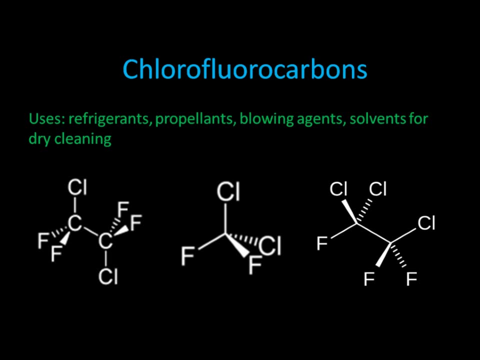 A single CFC is said to be able to destroy 100,000 ozone molecules. Why did we first create CFCs? CFCs were created as refrigerants, propellants such as aerosol sprays, blowing agents that create cellular-like frameworks in polymers and metals, and also for solvents used in dry cleaning.